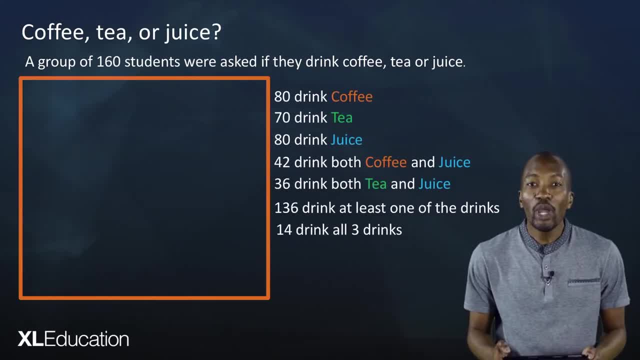 drinks. Now we must put all this information on a Venn diagram, But where do we start? Remember, 160 students were asked about these three drinks, So our sample size is 160.. Now we have coffee, tea or juice, meaning that we have three events. 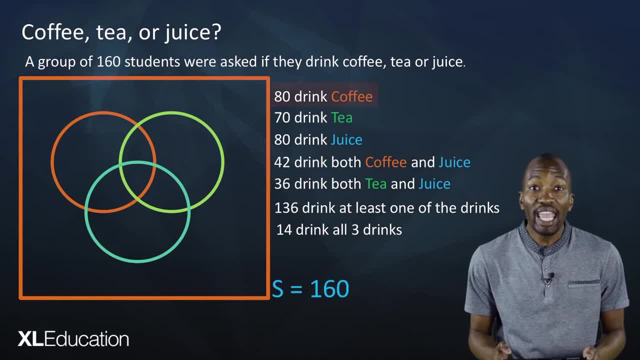 in our sample space, 80 drink coffee. So the circle for coffee is going to have 80.. We have a circle for juice. We have a circle for tea. We have a circle for juice, We have a circle for tea. We know that 70 drink tea, 80 drink juice, 14 drink all three drinks. What does this mean? 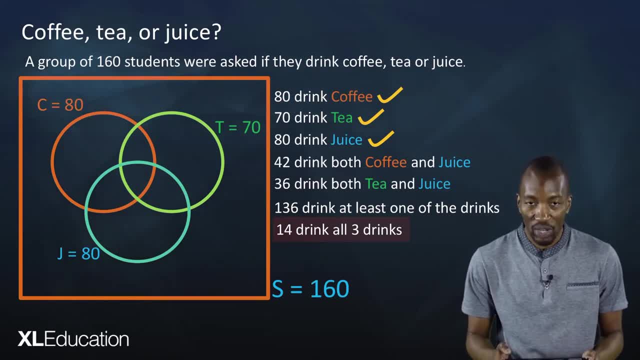 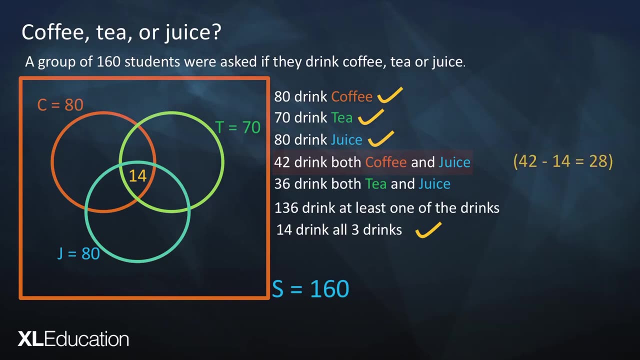 This is the intersection of all the three circles. So where all the three circles meet, we'll put 14.. Now, 42 drink both coffee and juice. This is the intersection of the coffee and the juice. But we already have 14 there. So how do we get the rest? We simply say 42 minus 14.. And this will 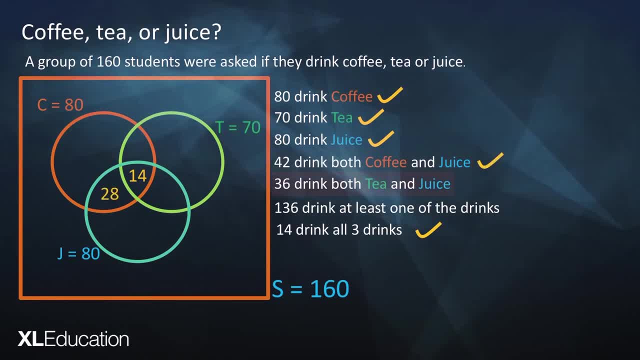 give us 28.. Now 36 drink both tea and juice. So we do the same thing: We take the 36, we subtract the 14 and we get 22.. Now 136 drink at least one of the drinks. So we do the same thing: We take the. 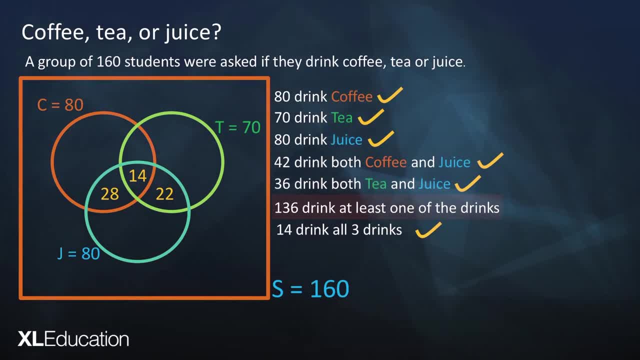 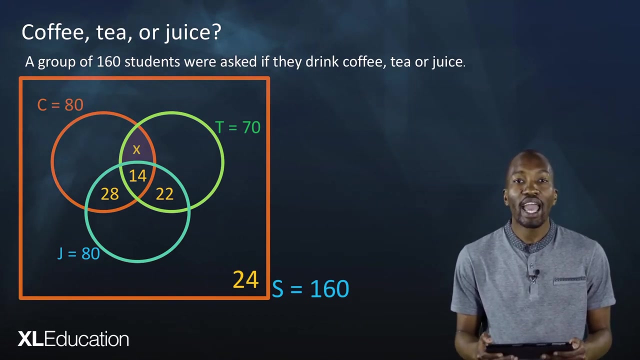 16 drink at least one of the drinks. This will help us find the number of people who do not drink any of the three drinks. How do we find this? We simply say 160 minus 136. And this will give us 24.. Now we do not know the intersection of the coffee and the tea. In other words, we do not know. 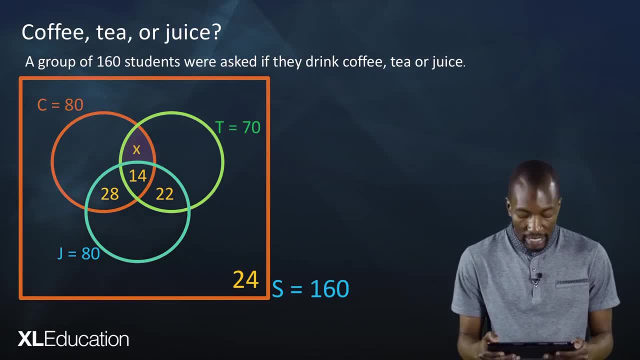 how many people drink both coffee and tea. So we simply say 160 minus 136.. And this will give us 24.. Now we do not know the intersection of the coffee and the tea. In other words, we do not know how many people drink both coffee and tea. So what will we do? We'll simply put an X there, because 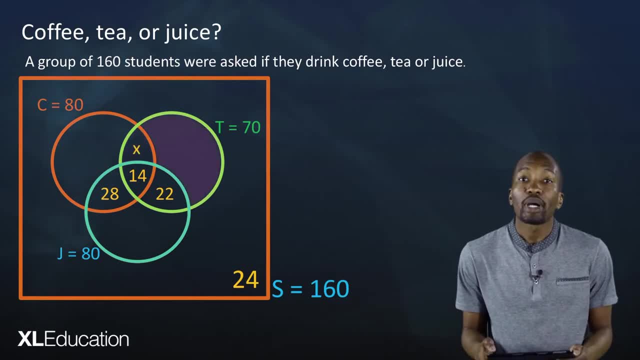 we don't know the number of people who drink both. But now how do we find the number of people who drink only tea? Remember, the number of people who drink tea is 70. So what we do is 17 minus 14 minus 22 minus X, And this will give us 34 minus X. This is the number of people who drink only tea. 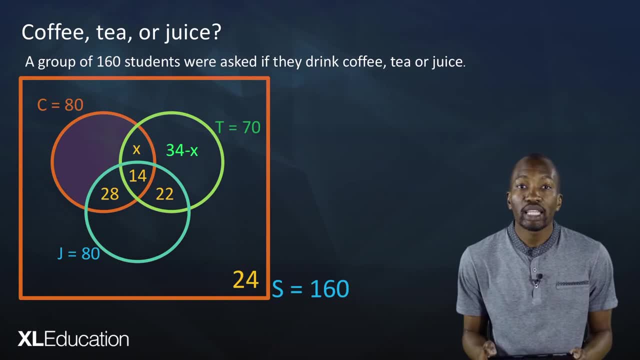 Now let's look at the number of people who drink only coffee. Remember, the coffee circle contains 80 people. So we'll do the same thing: 80 minus 28, minus 14, minus X, which will simplify to 38 minus X. This is the number of people who drink only coffee. Now let's look at the number of people. 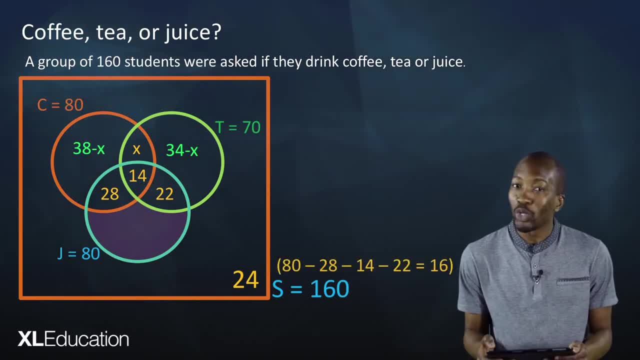 who drink only tea, And this will give us 34 minus 14 minus X. This is the number of people who drink only juice. We'll do the same thing here: 80 minus 28 minus 14, minus 22,, which will give us 16.. This 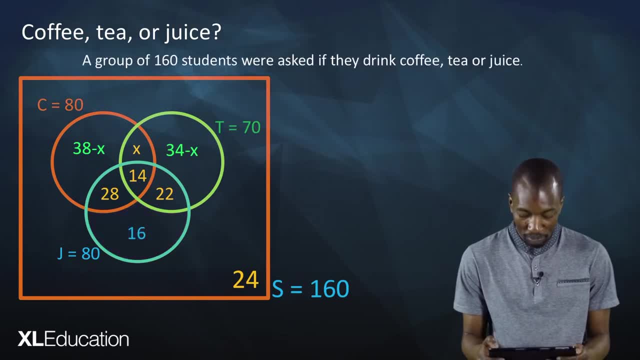 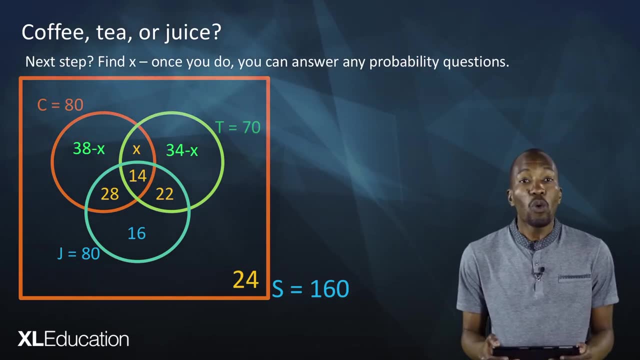 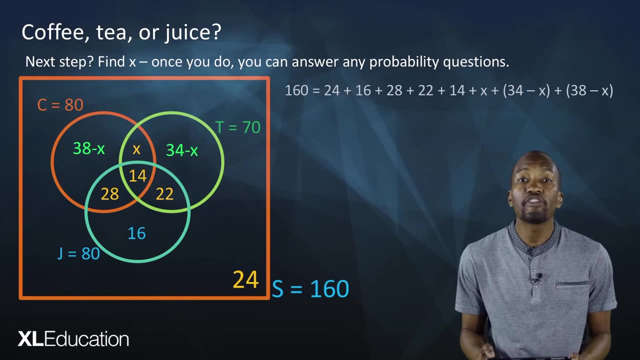 is the number of people who drink only juice. What is the next step? We need to find X. Once we find X, we can answer any probability question that follows. But how do we find X? This is very easy, because everything in our sample size added together must equal 160.. So we'll say: 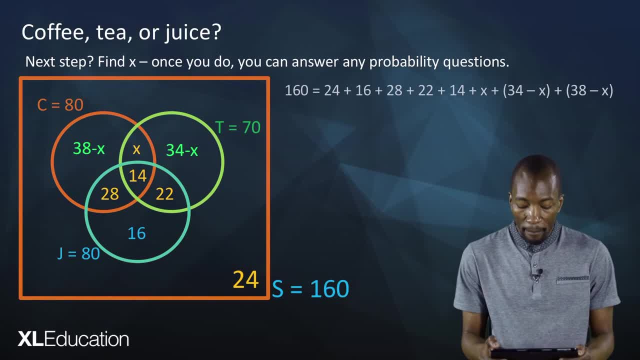 160 is equal to 24 plus 16 plus 28 plus 22 plus 14 plus X plus 34 minus X plus 38 minus X, And we'll solve for X. We'll get: 160 is equal to 176 minus X, And therefore X is equal. 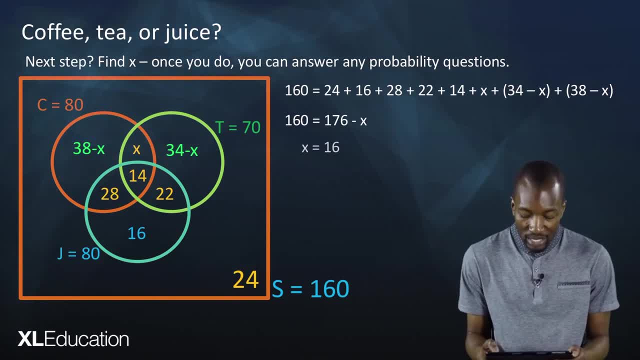 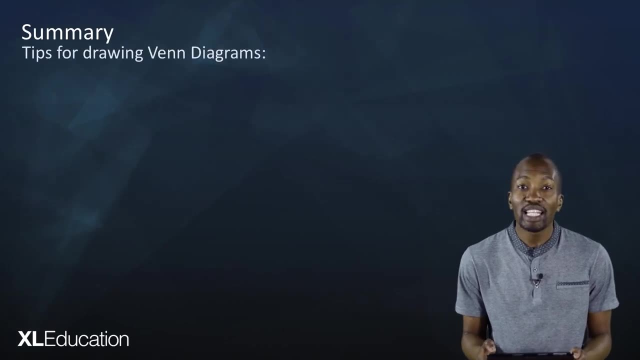 to 16.. Then we will replace X with 16. Then we know that the number of people who drink only coffee is 22.. The number of people who drink only tea is 18.. Now, in summary, let's look at the tips.